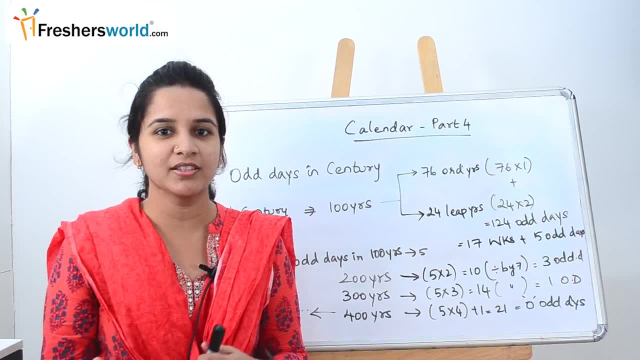 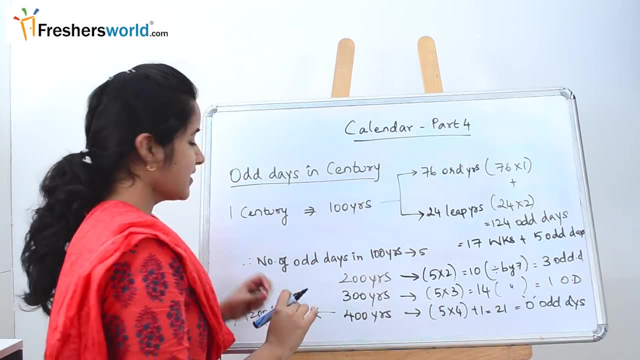 So in this case we will be talking about the sums that are falling under the topic of century. So let's understand this concept first. So let's talk about the odd days in a century. Let's take the 1st century first. 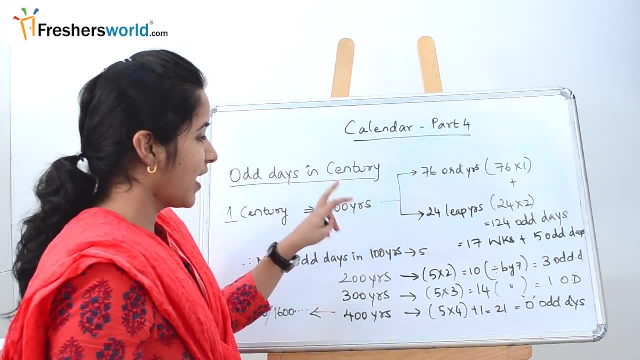 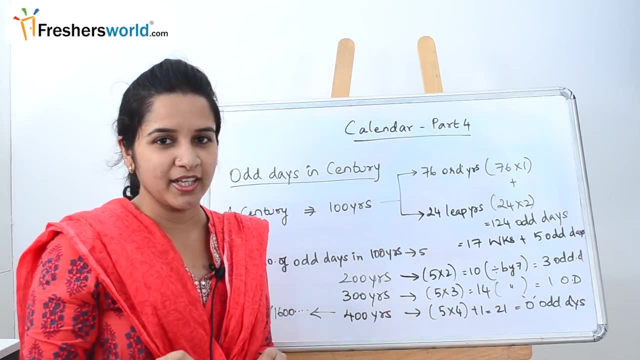 So 1st century is nothing but 100 years. So in 100 years there will be 24 leap years and 76 ordinary years. So we know in a leap year there are 2 odd days and in an ordinary year we have 1 odd day. 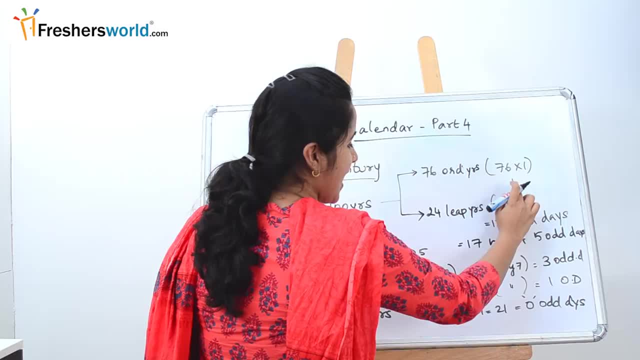 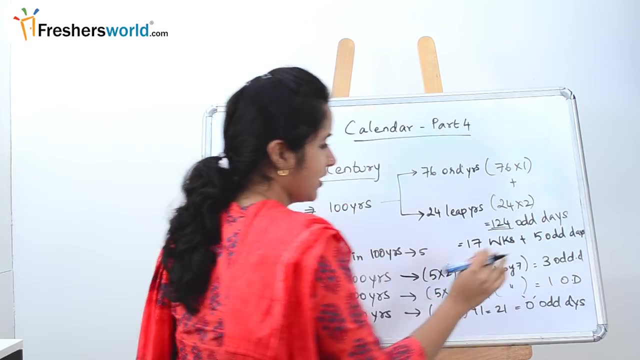 So what are we doing? We are multiplying 76 into 1 here and add it by 24 into 2, which is nothing but the 2 odd days. So once you multiply and add this, you will get 120.. So you will get 124 odd days together in a single century. 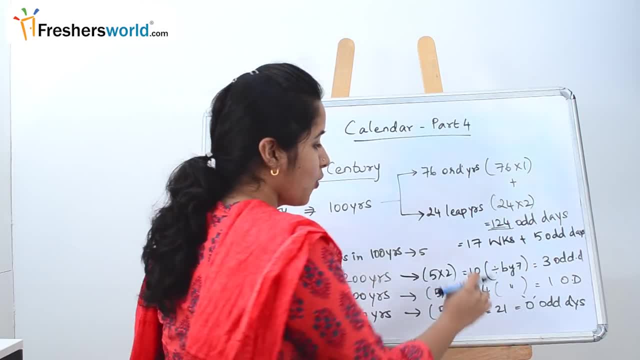 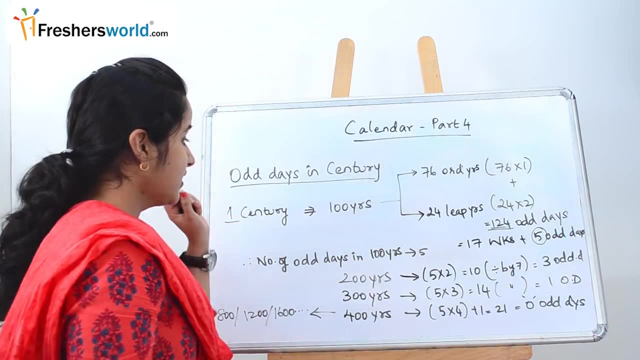 So 124 odd days. if you divide it by 7, in the quotient, you will get 17, and plus 5 in the remainder. So this 5 is nothing but your odd days. So in the 1st century, nothing but in 100 years, you will have 5 odd days. 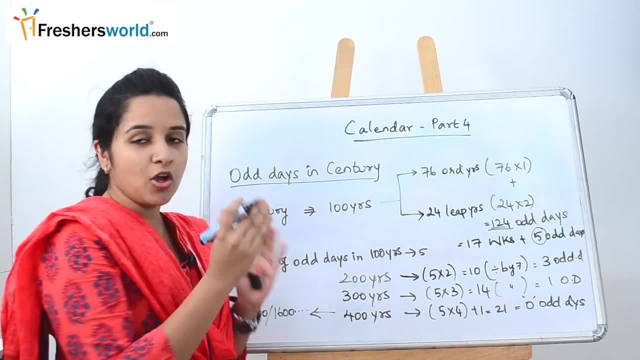 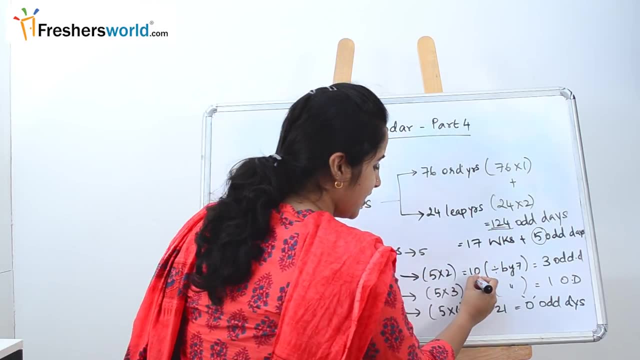 So, similarly, if you go for 200 years, the similar concept you are going to do for the 200 years. Instead of going and calculating all and all, what you can do is 5 odd days into 2, which is nothing but 10 odd days. 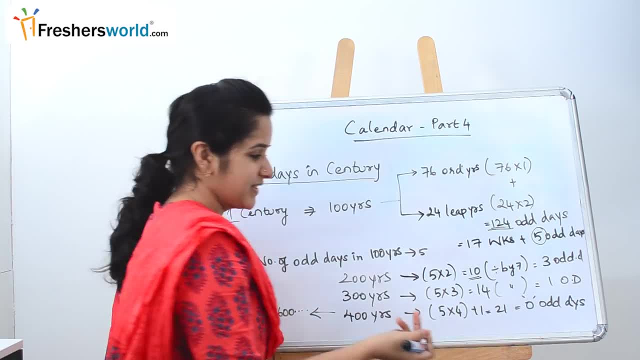 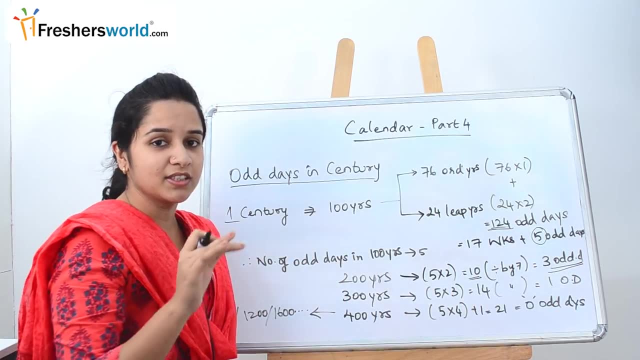 So what we are going to do here now is that we can again divide it by 7.. So if you divide it by 7, we know the remainder is 3.. So it becomes 3 odd days. So in 200 years we have 3 odd days. 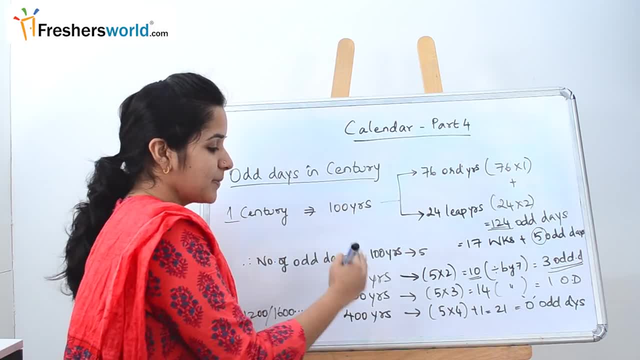 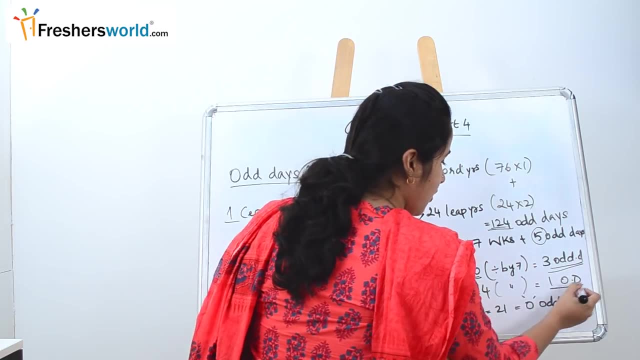 Similarly we are going to do for the 300 years. What do we do? We multiply 5 into 3, which is nothing but 15 divided by 7.. So the remainder is 1.. So in 300 years we have 1 odd day. 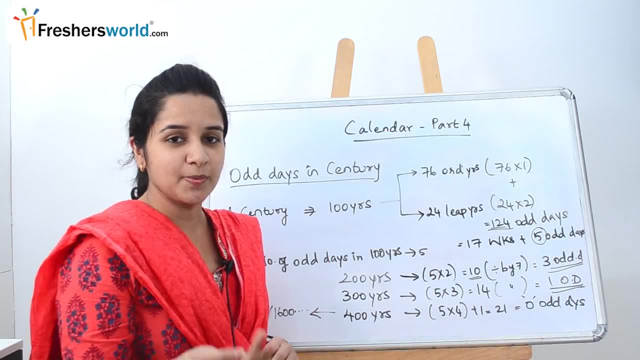 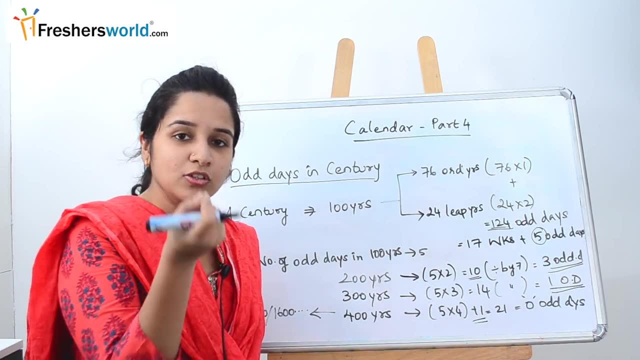 So in case of the 400 years, so as usual, we multiply it by 4.. So 5 into 4.. Why is this plus 1 here? Because every 400 years that particular year will also be a leap year, So we add this extra 1 odd day. 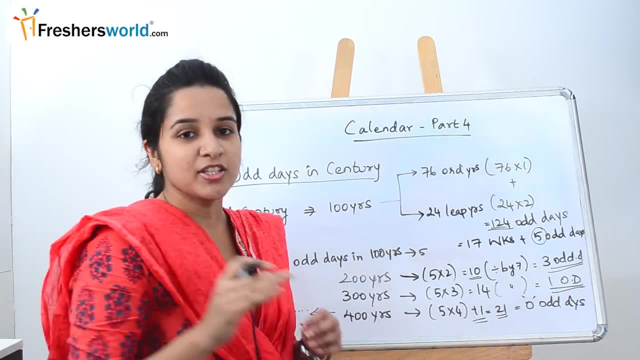 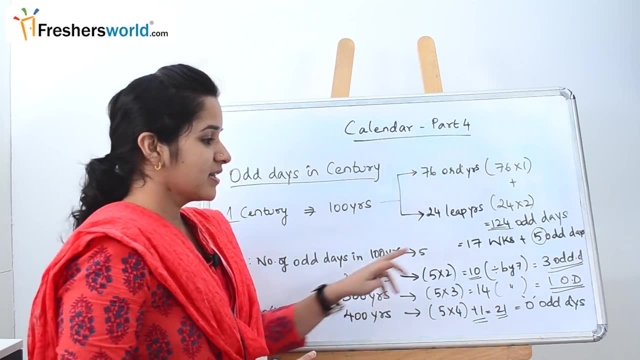 So it becomes 21.. So it becomes 0 odd days. So it's clear that in 100 years we have 5 odd days, In 200 years we have 3 odd days. To 300 years we have 1 odd day, and in 400 years we have 0 odd days. 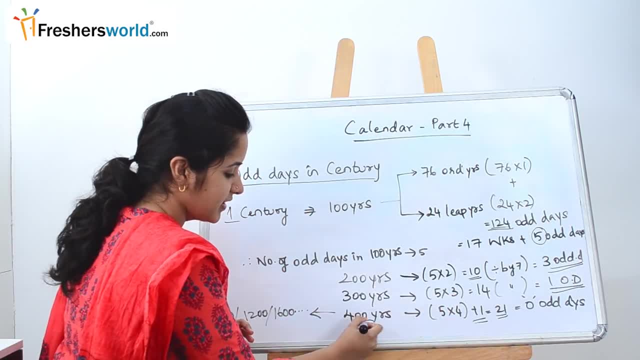 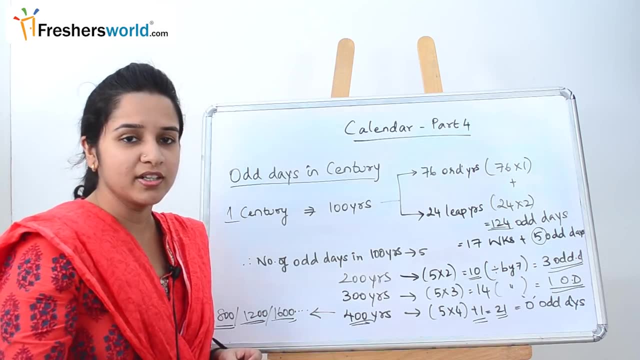 This whole pattern will be repeated This 400 years. 0 odd day will be repeated for the 800th year, 1200th year, 1600th and so on. For every 400 years there will always be 0 odd days. 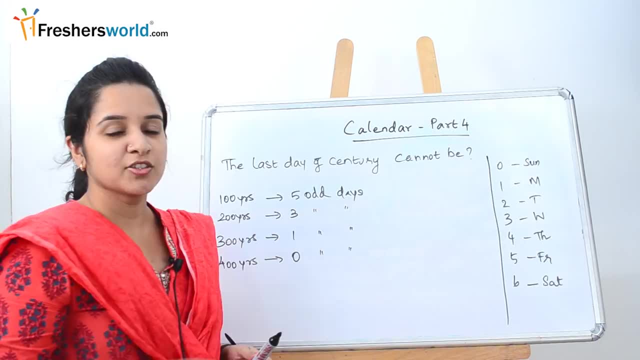 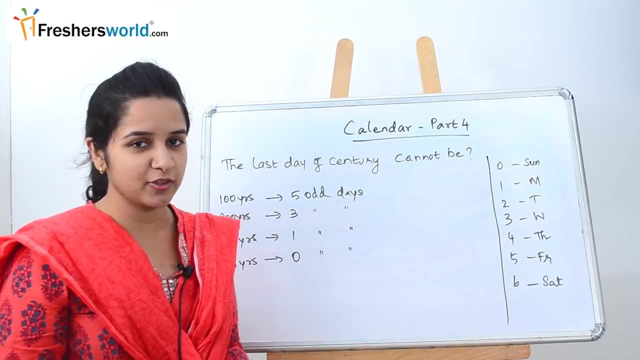 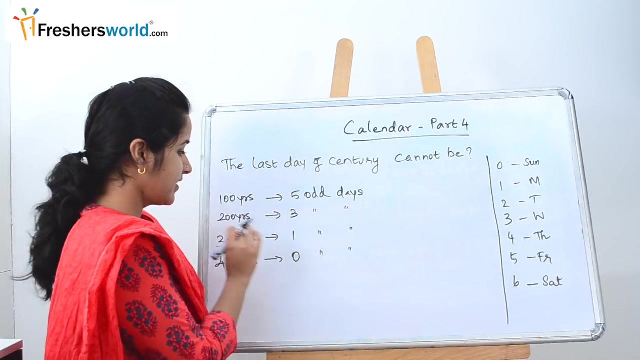 Let's solve couple of problems to understand this concept better. So the question that they have given is: the last day of the century cannot be So. there will be four options given to you. So how to solve this kind of problem. So how we start is that we know that 100 years have 5 odd days, 200 years have 3 odd days. 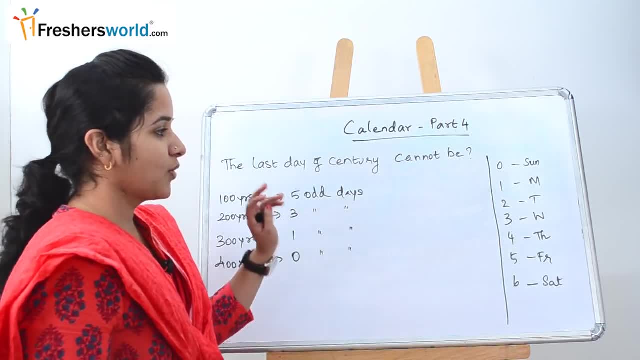 300 years have 1 odd day and 400 years is 0 odd day. So if you see, in the part 1 of the calendar we discussed about the coding of these days. So 0 to 6 is nothing but 5.. 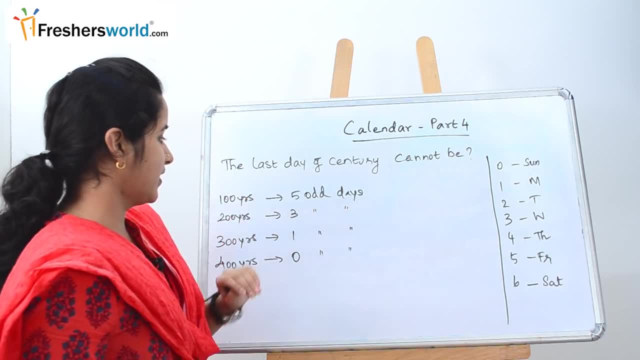 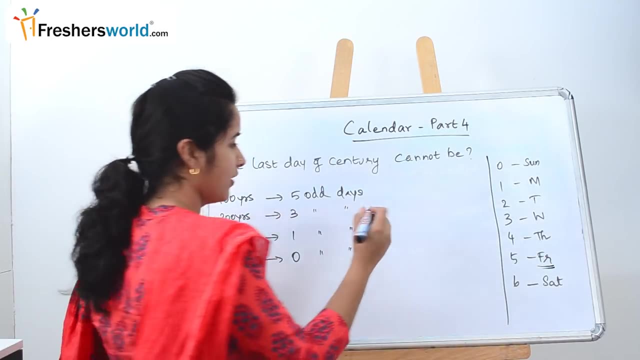 But from Sunday to Saturday. So 100 years have 5 odd days. So 100th year will have 5 odd days. 5 is nothing but Friday. So the 100th year day, final day, will be falling on a Friday. 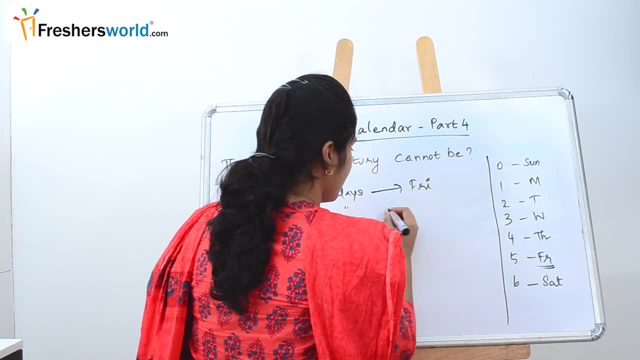 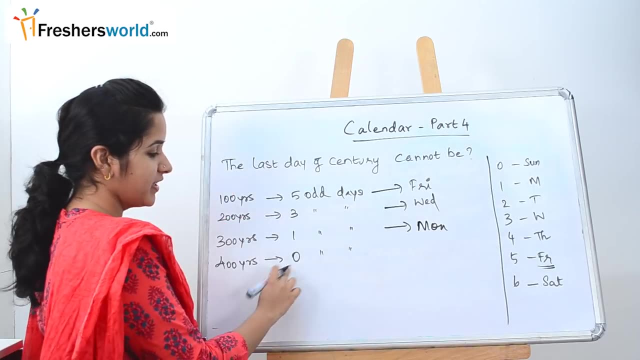 So 200 years has 3 odd days, So 3 is nothing but Wednesday. So 300 years will have 1 odd day, which is nothing but Monday, And 400 years will have 0 odd days, which is nothing but Sunday. So this cycle will be repeated for all days. 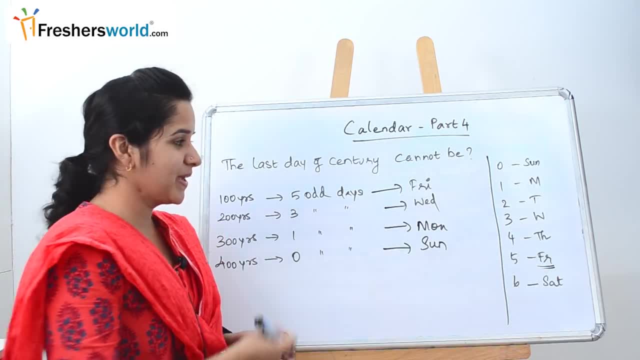 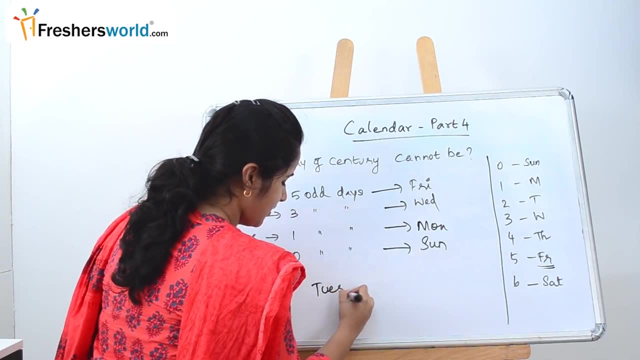 So this cycle will be repeated for all days. So repeatedly, you will see it will be either Friday or Wednesday, or Monday or Sunday. So what are the days that are left out? So Tuesday is left out, Thursday is left out and Saturday is left out. 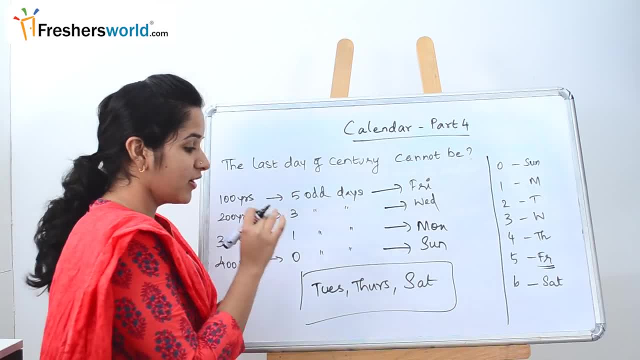 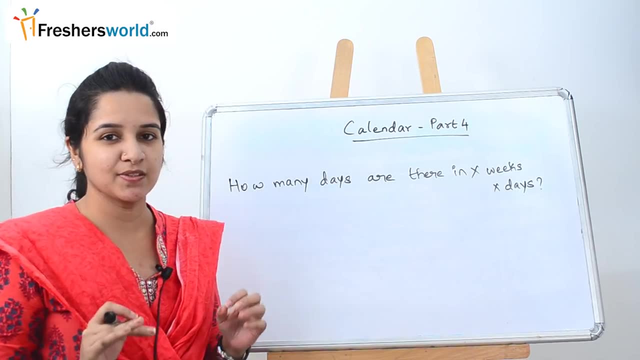 So the last day of the century cannot be a Tuesday or a Thursday or a Saturday, So lets solve another sum. So next question is: how many days are there in스 weeks and our days? How to find this 1 Number of weeks we have given? 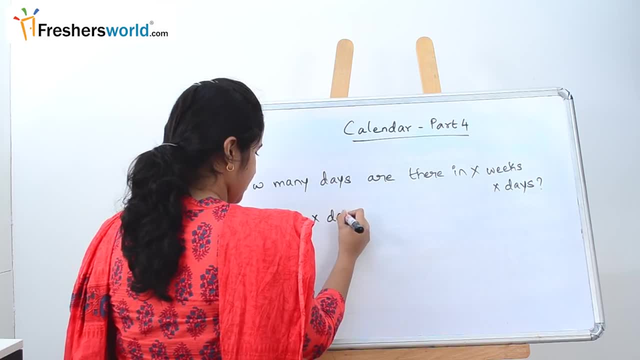 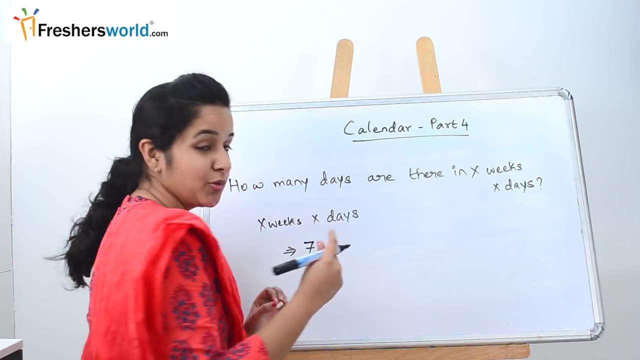 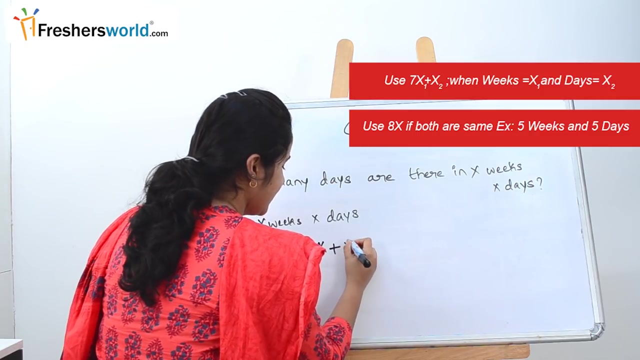 2, X weeks ready and x days. so we know that in a week there are seven days. so 7 into number of weeks. number of weeks is nothing but X plus the number of days we don't know. so we add it another X. so 7x plus X is equal to 8x. so sometimes they might give. 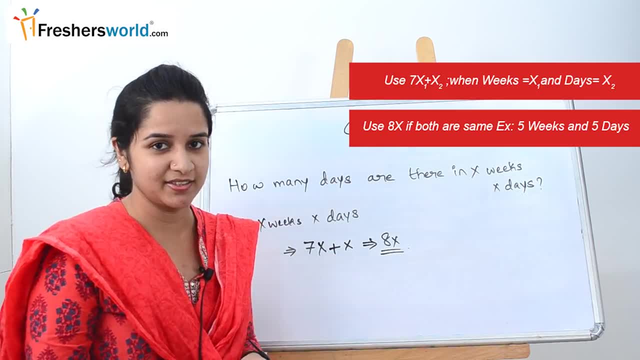 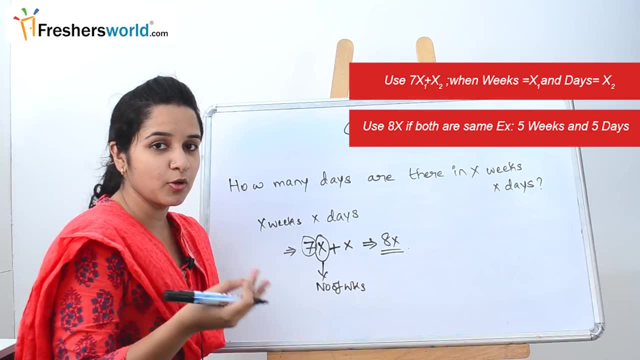 you a value in this X where you need to substitute and find the answer. so this shows the number of weeks that they have given in the question. multiplied by 7, 7 is nothing but the number of days in a week plus the anonymous number of days.